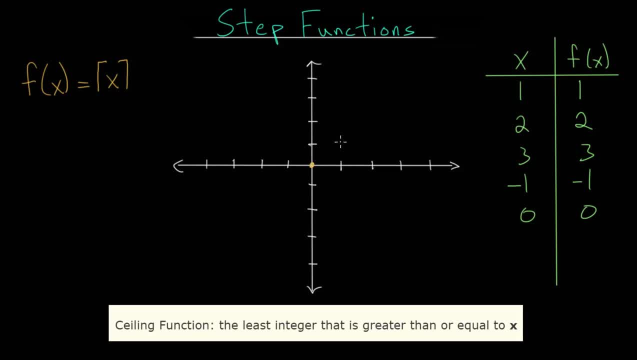 quickly. So we have the origin. we have it at 1, 1,, at 2,, 2,, 3,, 3,, 4,, 4,, 5,, 6,, 7,, 8,, 9,, 10,, 11,, 12,. 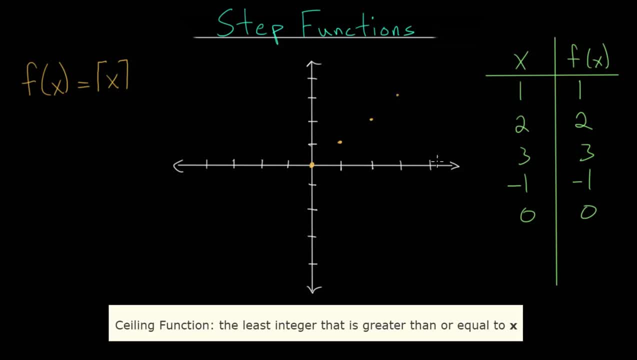 13,, 13,, 14,, 15,, 16,, 17,, 18,, 19,, 20,, 21,, 22,, 23,, 24,, 25,, 26,, 27,, 28,, 29,, 30,, 31,, 22,, 23,, 34, and so on. 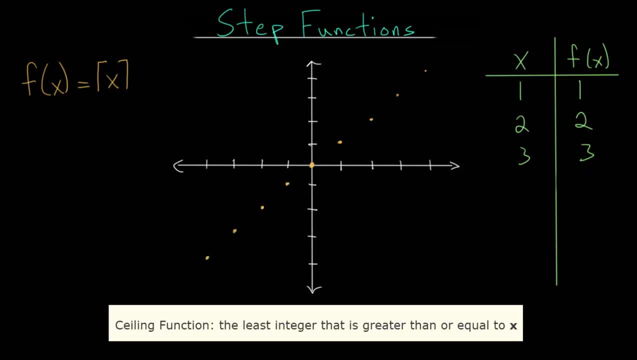 Let me just fill these in. So for integer values the function is not too exciting. It just essentially lines up. It almost looks linear. but when you start to get to fractional amounts it becomes a little bit more interesting. So let's say we plug in 1.1 here. 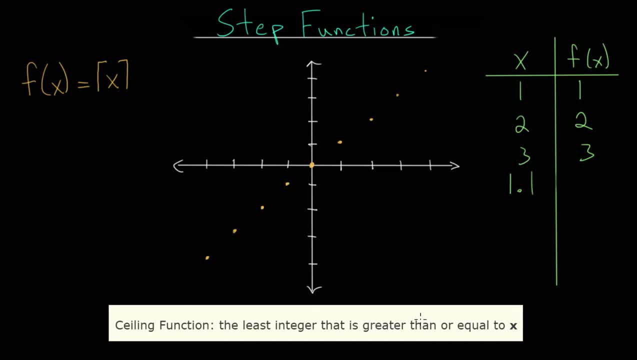 So the y value is the least integer that is greater than or equal to 1.1.. So there are many integers that are greater than 1.1.. In fact they're an infinite amount. So 2 is greater than 1.1,, 3,, 4,, 5, and so on. But we want the least of those, So the smallest. 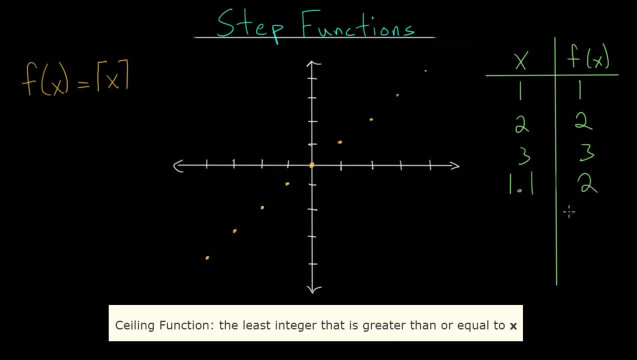 integer that is bigger than this number is 2.. In fact, one point: anything. for the most part, let's say 1.8, the least integer that's bigger than this is also 2.. So if we were, let's say: 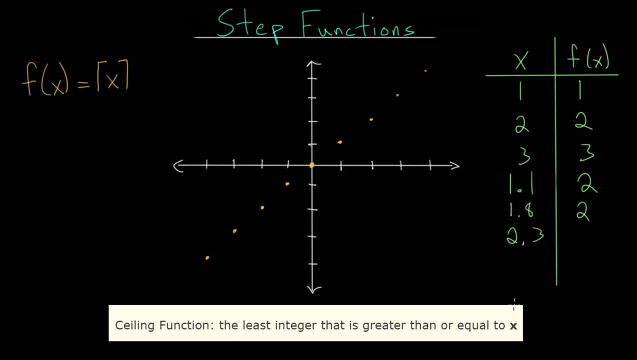 to look at 2.3, the least integer that's bigger than this would be 3.. And 2 point pretty much anything. let's say 2.99, the biggest integer that's bigger than this number is also 3.. 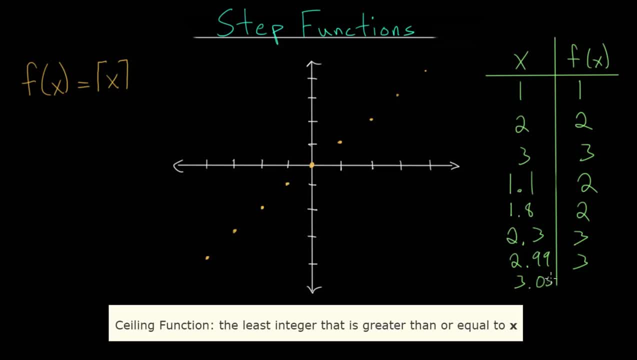 When we move up to 3 point- something, let's say, 3.05,, the biggest integer that is greater than this number is now 4.. So the way this function works is that whatever number you have, it will effectively round it up to that nearest integer. 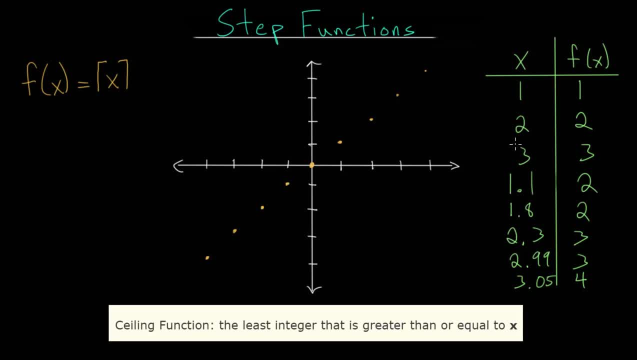 But if it is an integer, it's just going to remain that integer. So 1 point. anything is going to round up to 2, though you have to be careful When you have something like 1.9 repeating. so this is 1 point, something, but technically, 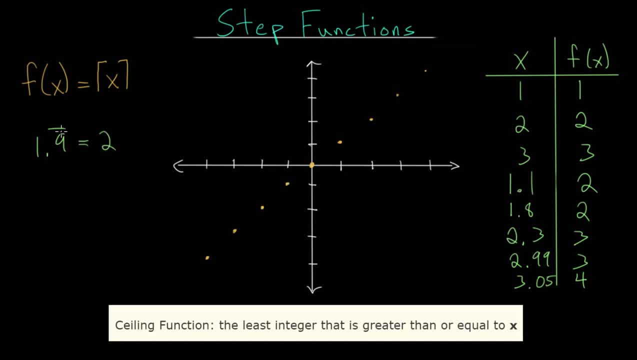 this is equal to 2.. So if it's an infinite string of nines after the decimal, it does equal the integer above that. So, and that would be true for 2.9 as well, 2.9 repeating that's also equal to 3.. So that's the only point of contention there. But technically, 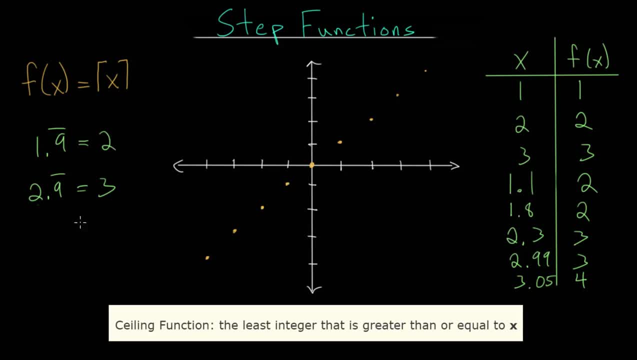 this is not less than 2,, this equals 2. And likewise for this one as well. So if we start trying to graph our picture here of this C-link function, let's look at x values between 1 and 2.. So when x is equal to 1,. 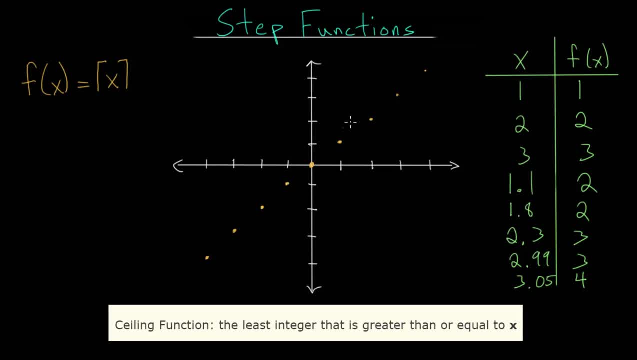 the y value is 1.. But when x is 1 point, something that is slightly bigger than 1, the y value is going to be 2.. So it's not going to include that point, Since when x is 1, it's 1.. But for anything that is slightly bigger than 1, it has a y. 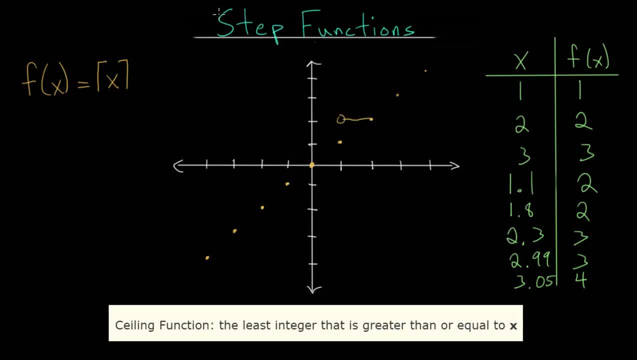 value of 2.. And then we're just going to get a flat line or a horizontal line here going across, And likewise between 2 and 3. The y values are going to be at 3. Except for this point right here, when x is actually equal to 2. So for x values that are slightly bigger, 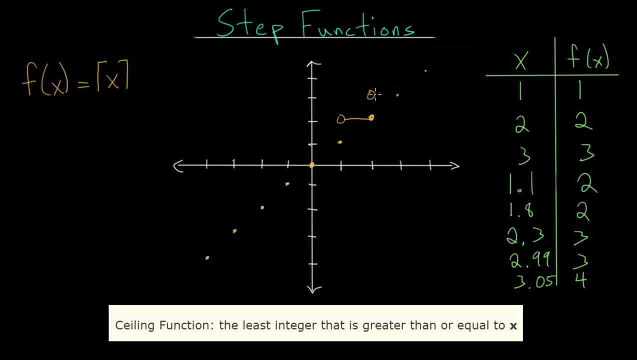 than 2.. So we use an open circle to represent that The y values are gonna be three and they end here, And when x is slightly bigger than three, the y values essentially get rounded up to four. But again, it's not including that point. 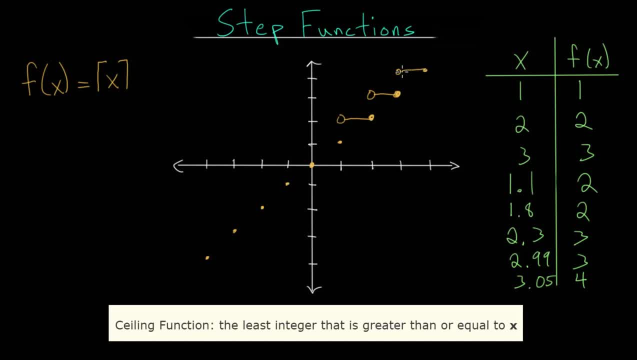 so we use another open circle and then another flat line to represent that all points not including three, but going all the way to four and including four, all those x values return a y value of four. So it looks just like our other step function. 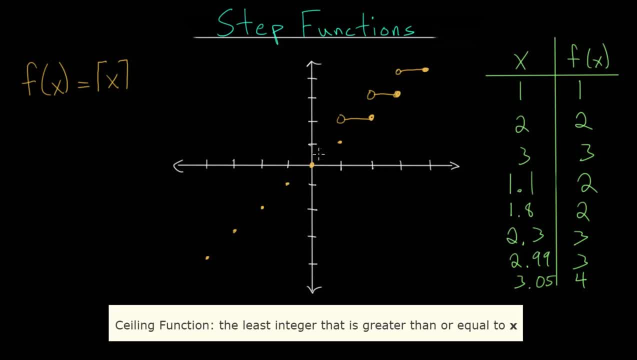 our floor function. but compared to that, everything is shifted up one unit. So between zero and one, not including zero. the y value is at one, between negative one and zero, not including negative one. So we use that open circle.